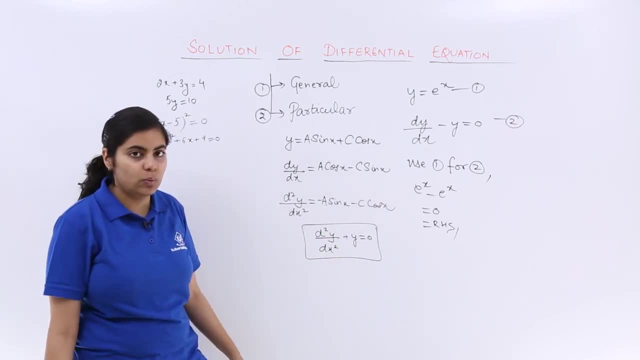 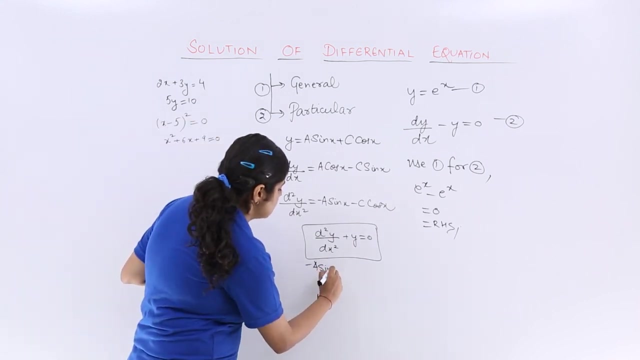 the given differential equation: Does y is equal to a sin x plus c cos x satisfy this differential equation? Yes, definitely, because d2y by dx square value we are going to put which is minus a sin x, minus c, cos x, right plus y. So plus y is plus c cos x Is anything. 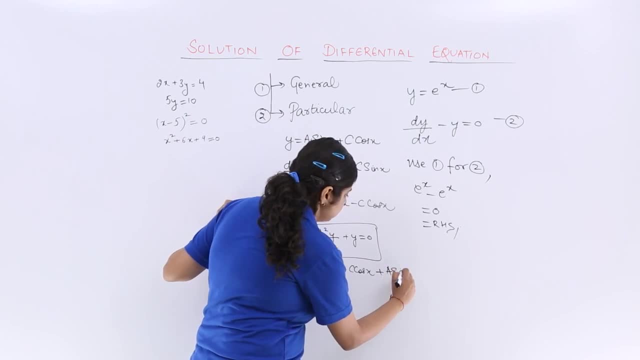 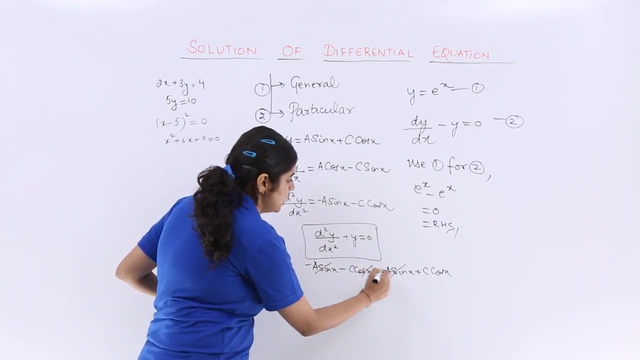 wrong. Are you happy? Yes, Why? You have more solution than mine. Then you are right. a sin x plus c cos x. now these two are put. let's see if something cancels. these two things get cancelled because of the opposite sign and equal magnitude, so it becomes equal. 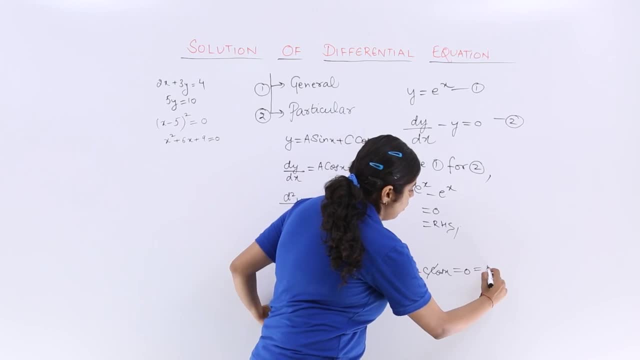 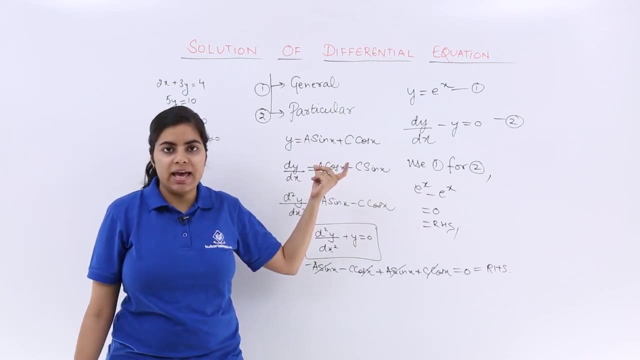 to 0 and 0 is equal to 0, which is RHS. so what do you know? we know that definitely a sin x plus c cos x is there, and that is the solution to this given differential equation. right, because it gave me, left hand side is equal to the right hand side. but what kind of a. 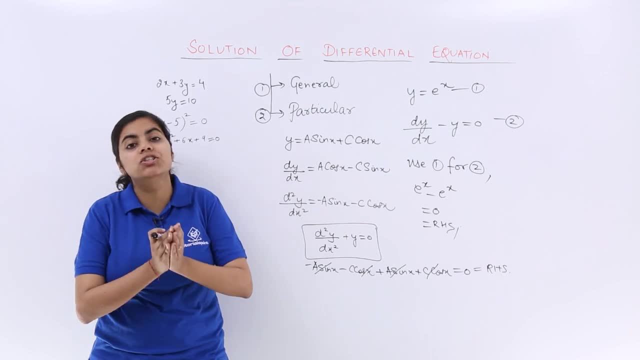 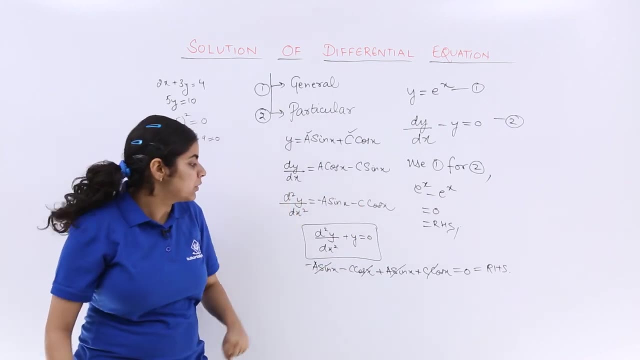 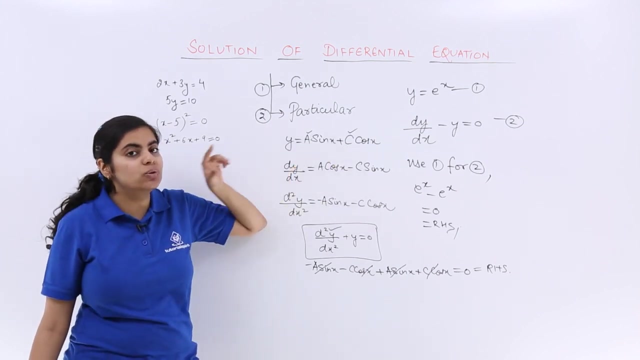 solution is this. this is what kind of a solution? a general solution, because, see, the number of constants were a and c, which were two arbitrary constants. the final order of the differential equation is also two and there is no particular value assigned to these arbitrary constants. so this is the general solution. 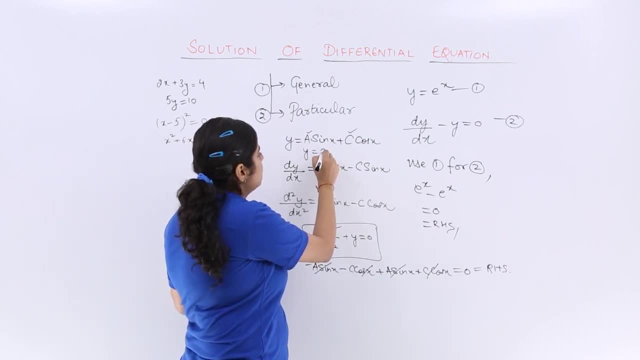 But if you want to know how to solve a differential equation, then you need to know how to solve a differential equation. So if I say that this time it is y is equal to say 3 sin x plus 8 cos x, and then I solve. 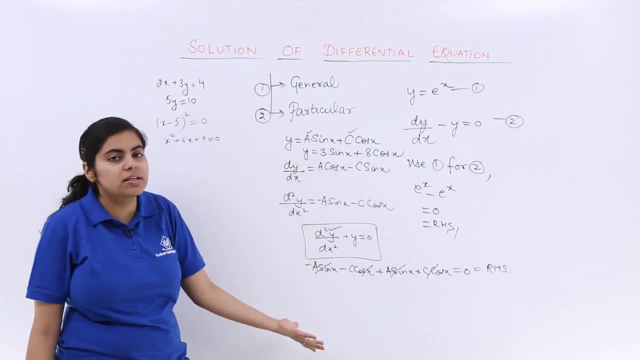 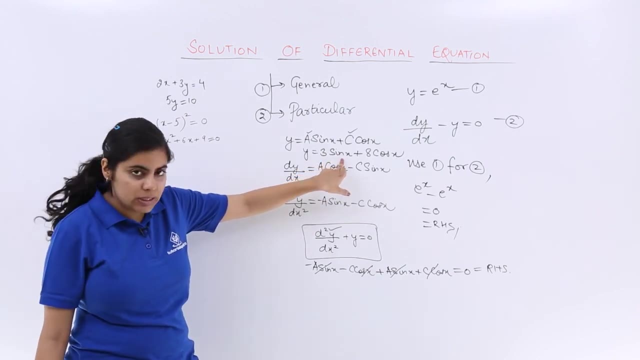 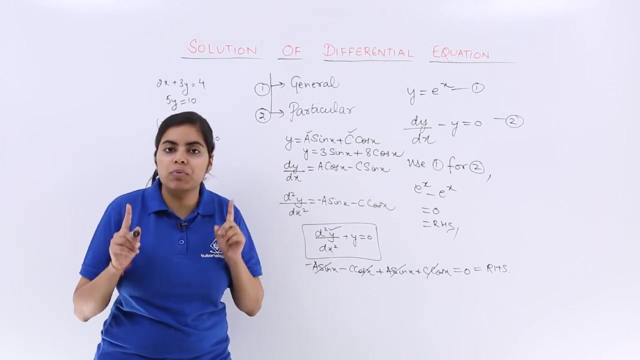 it again. I will get something called as 0, because differentiation is irrespective of the value of the constants. so that means I say that y is equal to 3 sin x plus 8 cos x is the particular solution, not the differential one. why? because I know that the particular 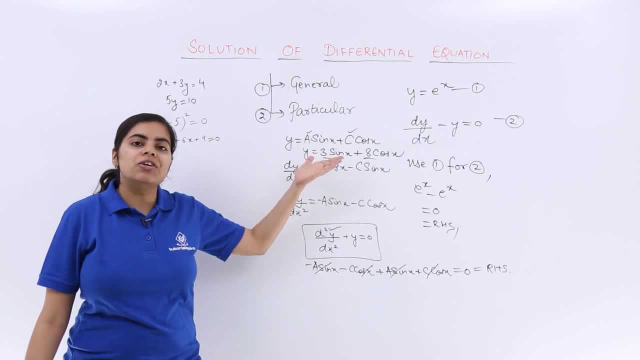 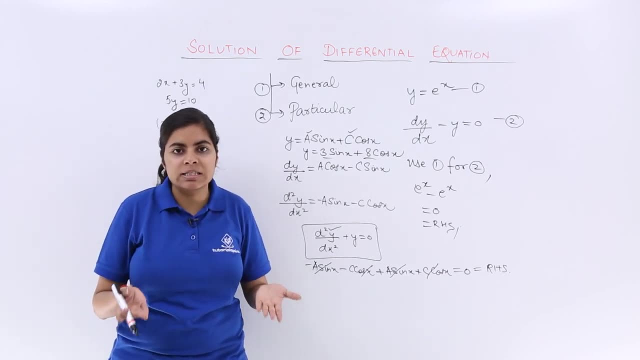 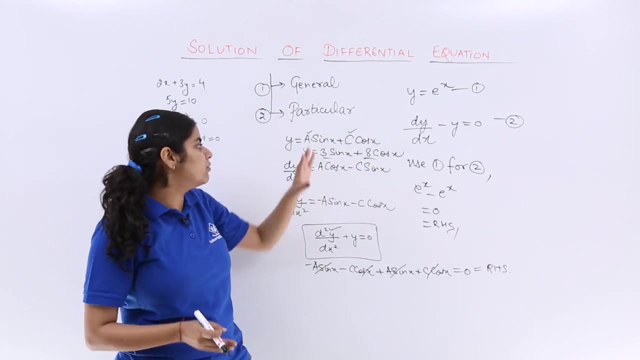 solution has a particular value assigned to the constants. general solution does not have any particular value assigned to the constants. particular literally means what specific right. so specific value assigned to the arbitrary constants gives me a particular solution, while the above one is giving me a general solution.